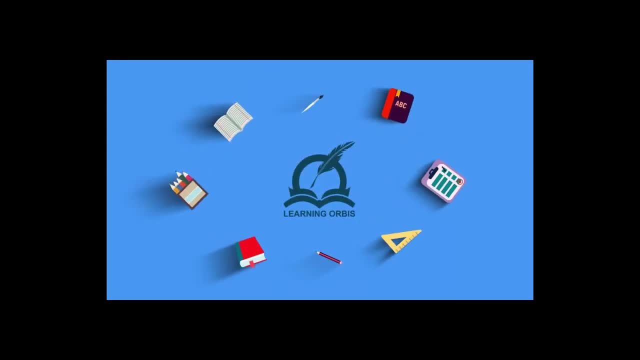 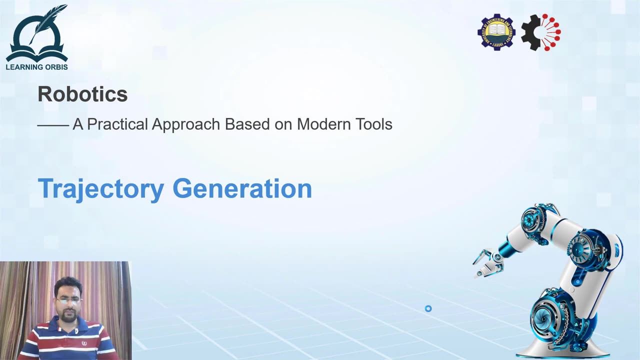 Assalamu alaikum, Dear learners, I hope you are fine and doing well. In the previous couple of videos we have seen that how we can simulate robotic manipulators in MATLAB's environment. We have studied that, what forward kinematics is and what inverse kinematics is, And specifically 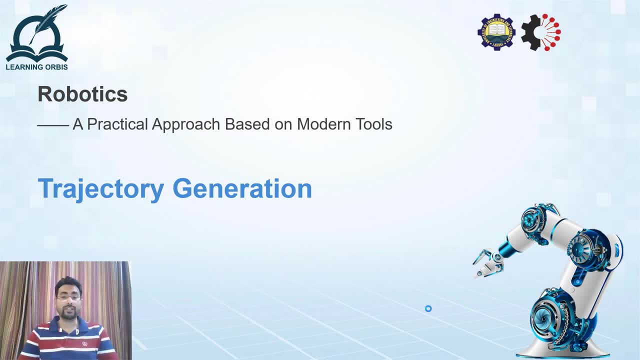 in the previous video, we generated a trajectory so that a robot can draw a square in its workspace. In that video, the trajectory that we created was completely manual, That is, we defined that at what time the robot should be, at which point And between any two points the robot was moving. 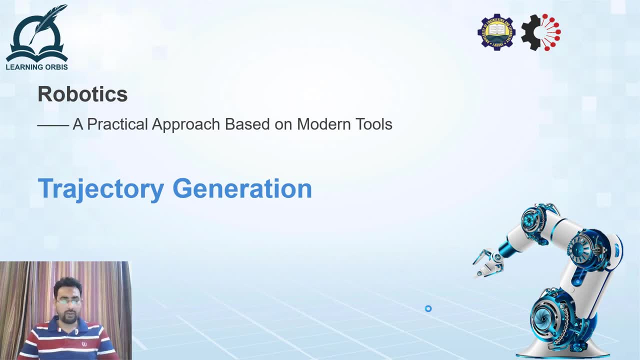 in a straight line without any regard to acceleration or velocities involved. However, in practical situations, controlling the velocity and accelerations are quite important, And therefore we should be considering these two things whenever we are generating the trajectory In Robotic System Toolbox. there are a couple of tools that can help us to generate a reliable 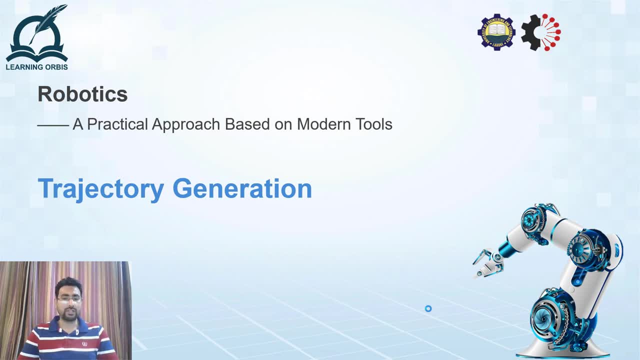 trajectory that will consider the accelerations, the end times, the velocities and other aspects of trajectory as well. So in this video we are going to see two of the function blocks that are available in Robotic System Toolbox that can be used to generate trajectories as per our wish. 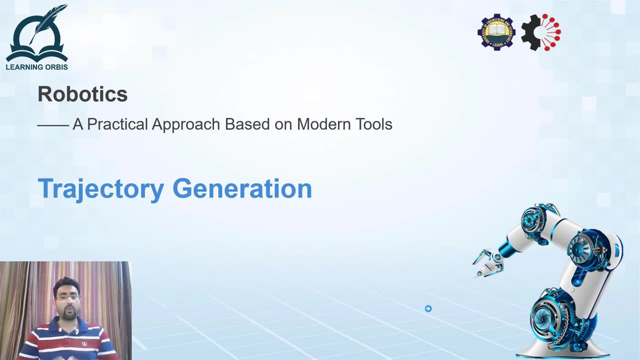 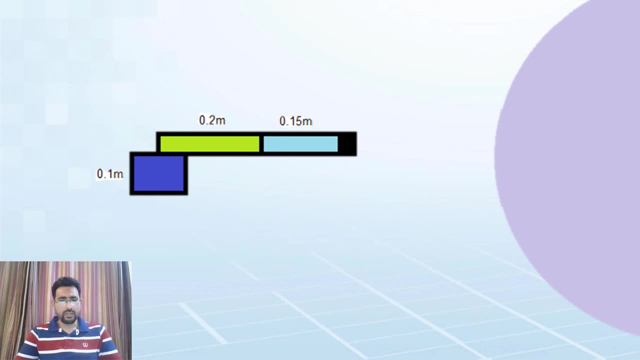 But before that, let me quickly recap that what we have with us and what we wish to do. So this was our robot, which is a planar, two-link, two degrees of freedom robot, And it cannot move in the z-axis but its end effector can move in x-y plane And it can go. 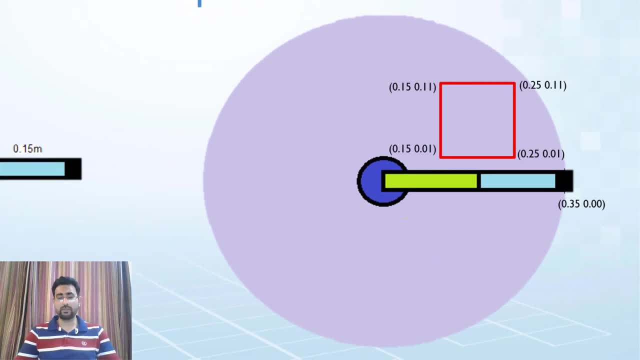 at a distance of two degrees of freedom, And it can move at a distance of two degrees of freedom At any point which is within the workspace of this robot. The workspace of this robot is shown by this gray area over here, And in the previous video we wanted the end effector to trace this. 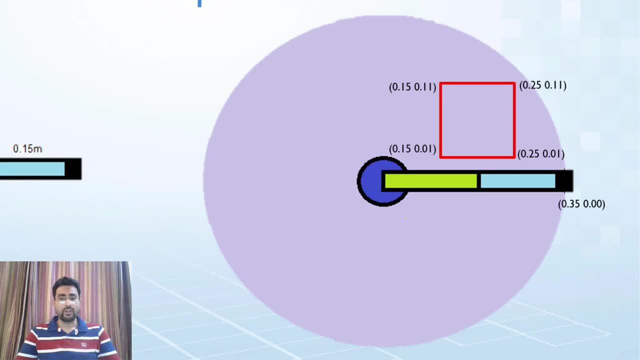 red square. So we provided the coordinates and the time values to a signal builder block that created a trajectory And the end effector moved on that trajectory. Note over here that there are going to be six waypoints which this end effector is going to follow. By waypoints I mean that the 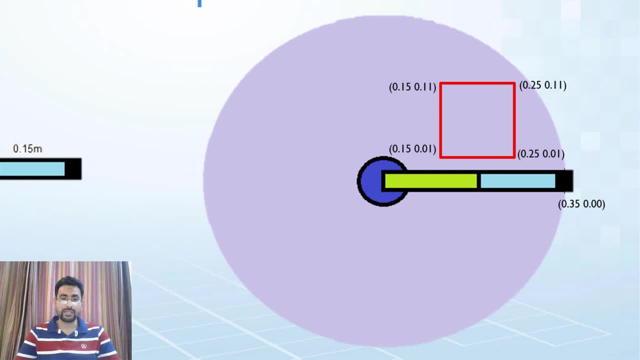 point in the workspace through which the end effector should move or should pass whenever it is moving. These six waypoints will be the initial point, that is, this point, then the four corners of the square and the last corner once again, because when we will go towards the fourth corner, then we have to return to the first corner at the end to complete the square. 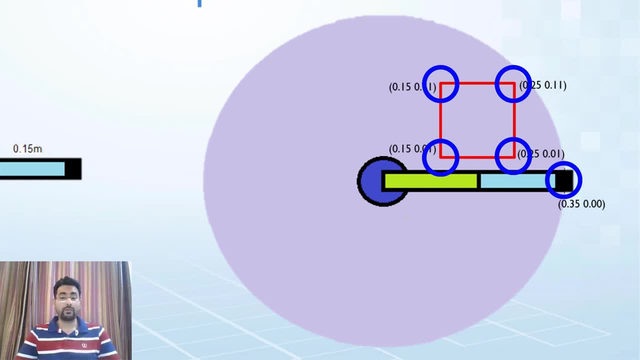 So there are going to be six waypoints And for the six waypoints there are going to be five trajectory segments. Now, to efficiently draw the square and to consider the velocities and accelerations while the robot is moving on this trajectory, we need to control certain things in all the trajectory segments. 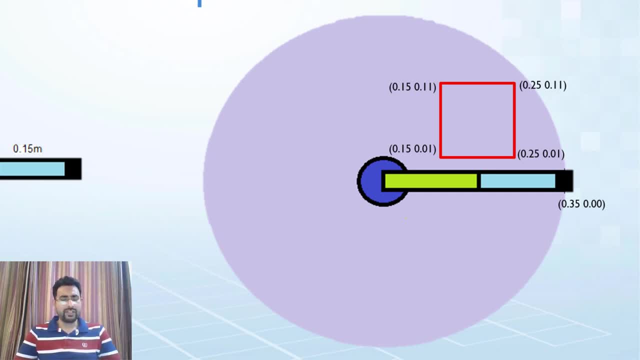 For example, one thing that we can do is we can approach the first square very carefully. Let us take a longer time to reach at the first corner, And once we have reached there, then we move in a much speedy fashion. The things normally associated with trajectory generation are the velocities and the accelerations through which the end effector should move. For example, if you wish that at every waypoint the end effector should have a minimum velocity of, let's say, 0.1 meter per second, then you should be able to appreciate that you cannot, say, move at a maximum velocity of, say, 0.1 meter per second, L Night Per Second. 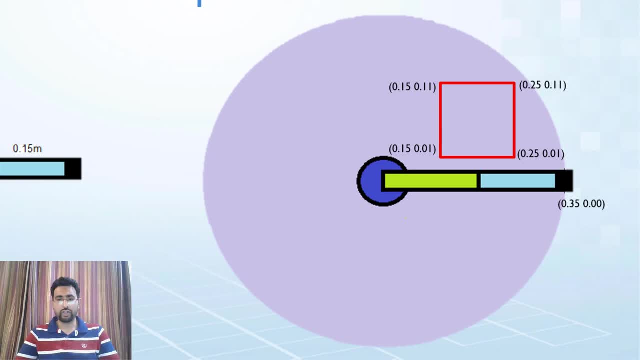 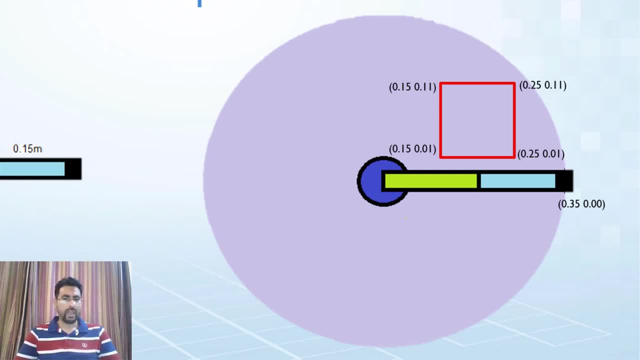 then, at each and every waypoint, the velocity should be 0. And if it's not 0,, then we cannot arbitrarily change the direction of end effector abruptly. Moreover, to speed up the process, the trajectory generation blocks of the robotic system toolbox. 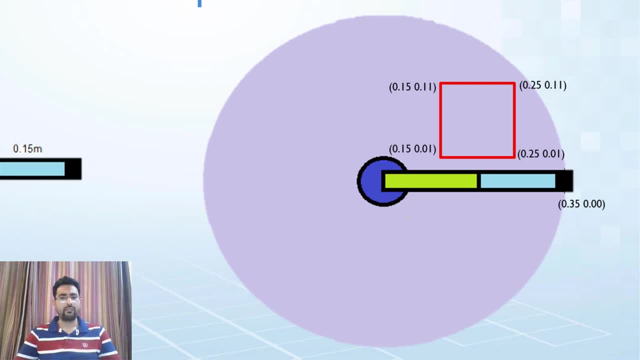 provide us with different details and different options so that we can readily generate the trajectory without worrying about the tiniest details of time and other things. So let's move on to the Simulink environment and check that. what are these two function blocks that we are going to use today and what we can do with them? 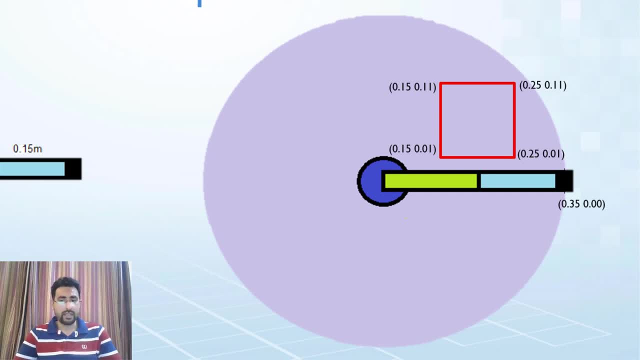 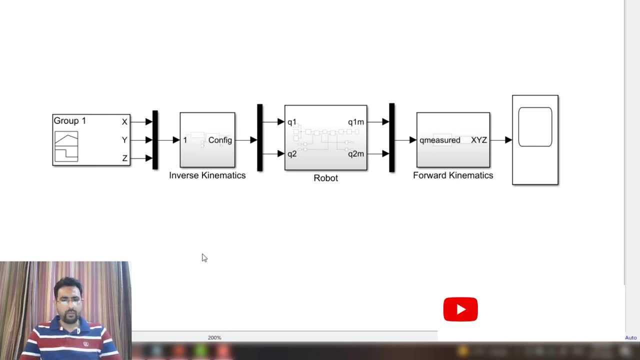 Can they generate the square which we want, Or do we need something else as well? So this is the Simulink environment And, if you remember from the previous video, this was what we created in that video. We used a signal builder to generate a trajectory. 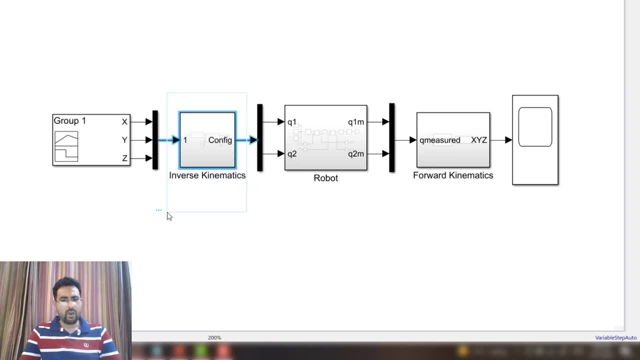 That trajectory was given to the inverse kinematics block. Inverse kinematics block generated the joint angles that were required for the robot to move And the robot moved on those joint angles. We measured those joint angles, provided those angles to the forward kinematics block and that block. 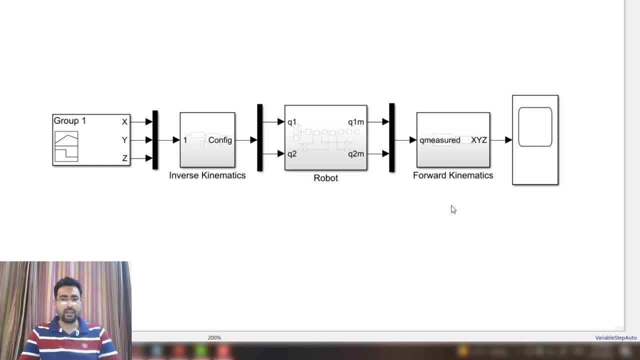 gave us the xy position of the end effector which we provided at the start over here. So this time around we are not going to use this signal builder, but in fact we are going to generate trajectory using the blocks from the robotic system toolbox. 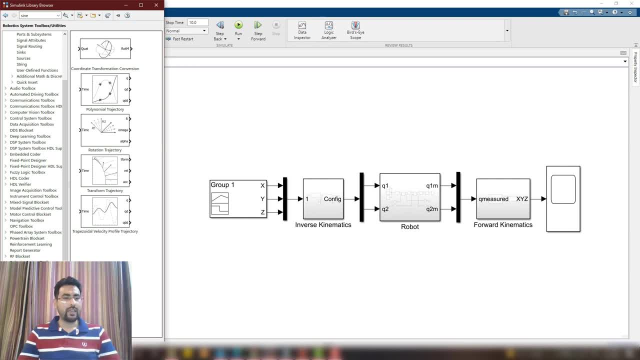 So in the robotic system toolbox and then in the utility section, we have four different blocks that can be used to generate trajectories. Out of these four, we are going to do two of them. The first one, which we are going to do, 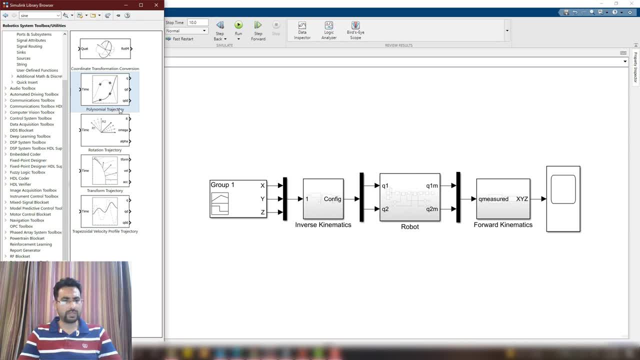 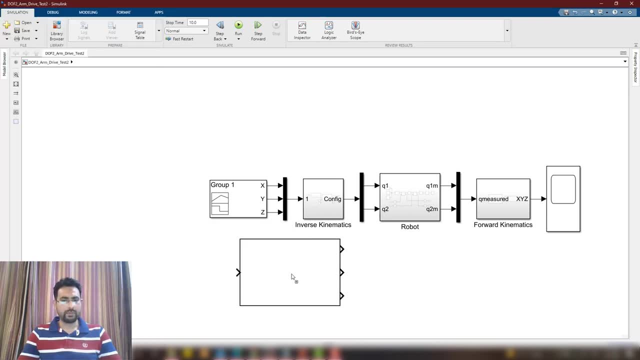 is the polynomial trajectory, And the second one that I'm going to discuss is the trapezoidal velocity profile trajectory. So let's start with the polynomial trajectory. Just drag this block to place it in your signal model. In this model, we don't need this thing. 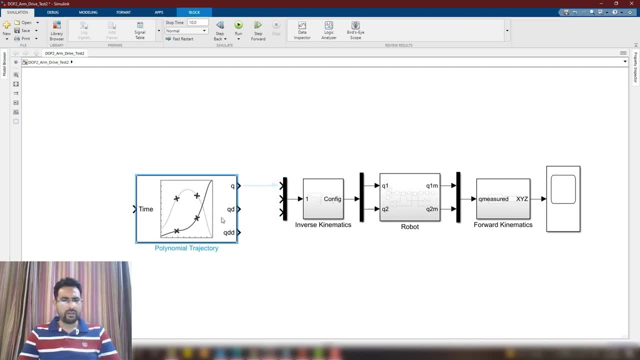 so I'm going to delete it. One thing you should be readily aware is that this block is going to generate three things. The first thing is the trajectory coordinates, The second thing is the velocities And the third thing is the accelerations. Be advised that Q over here doesn't mean joint. 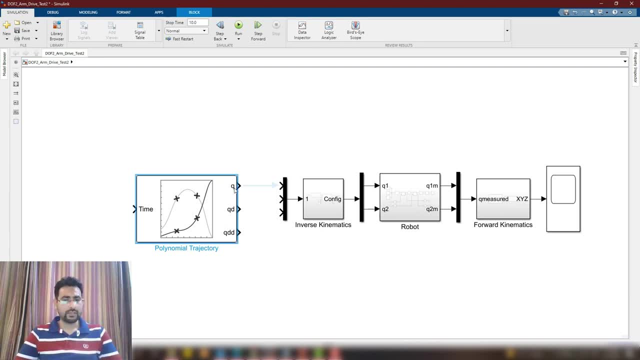 Q represents the x, y, z position of the trajectory. So these are just x, y, z locations. Qd would be the velocity in x, y and z direction, whereas Qdd is the accelerations in the x, y and z directions. 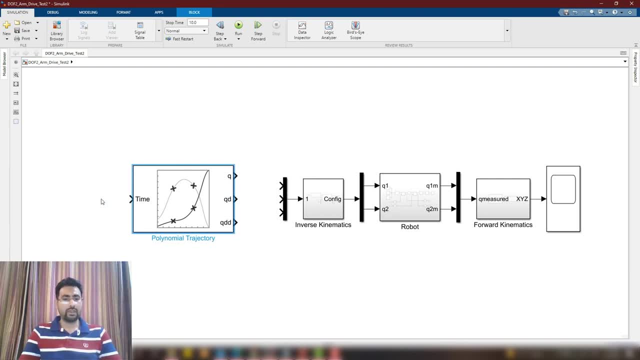 The only input that this thing requires is the time, because trajectory needs time. So I'm going to place a clock over here that will supply time to this block. And then we have to configure this block by going into its properties, Coming into the properties, the very first thing over here. 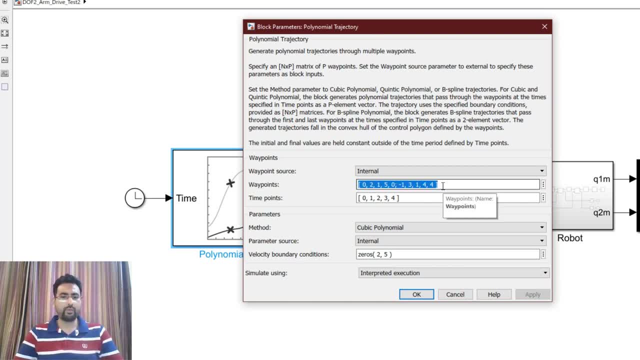 is the weight We need to supply, the weight points through which we wish our end effector to move. So, using our example of tracing a square, weight points would be these ones. I have already stored the weight points in the workspace under a variable named wp. 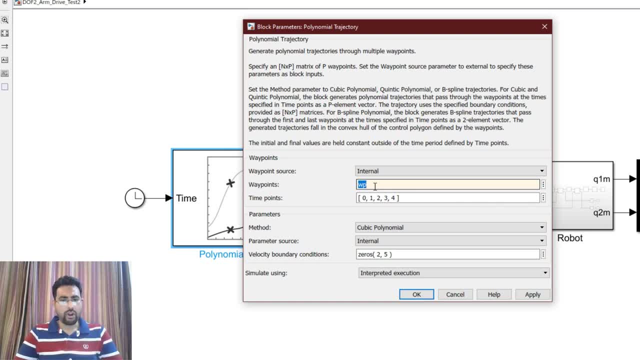 We advise that this block requires weight points in an order of n cross p, where n is the number of x's. That is, we have x, y and z x's. Therefore, the number of rows would be three And p represents the number of weight points. 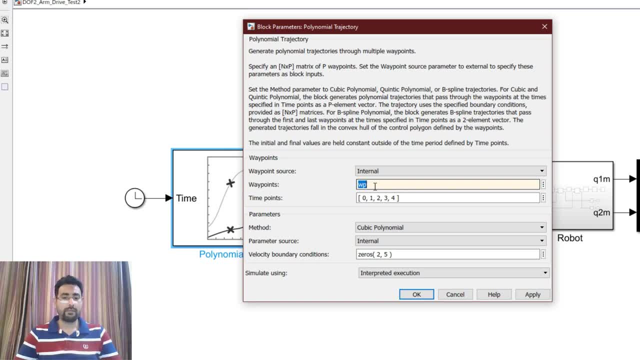 So we had six weight points, so I have arranged them in this order and placed them in the variable wp and have supplied that variable over here. So the second thing we need to give is the time points. As we have six weight points, we need to give six time points. 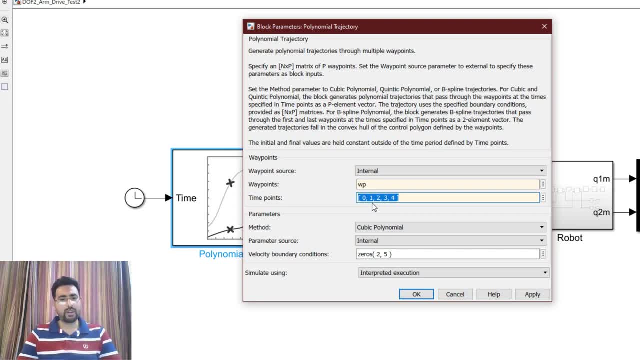 That is, at what time the end effector should reach at a particular weight point. So we want the first weight point to be reached at 0, because it is the initial weight point, And the second weight point, which would be the first corner of our square. 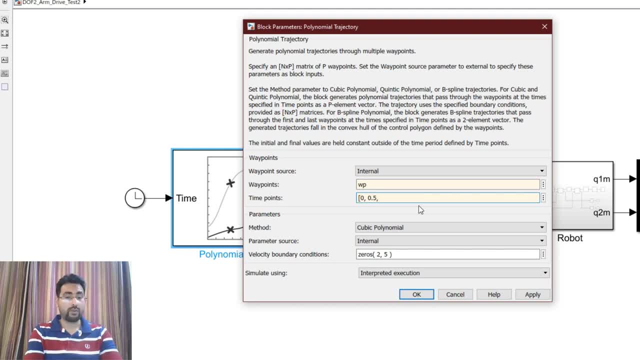 should be reached by 0.5 seconds, And after one second I want my end effector to reach the second corner of the square, So I'm going to input 1.5.. That is, it will take one second to go from the second weight. 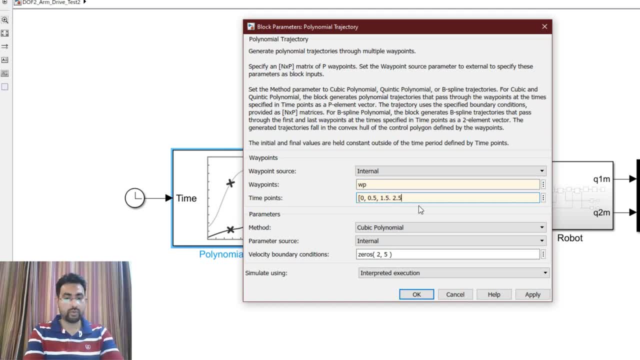 point to the third weight point, Then I need one more second to go to the third corner of the square, then one more second to go to the fourth corner of the square and then at the end I want the end effector to reach the first corner once again. 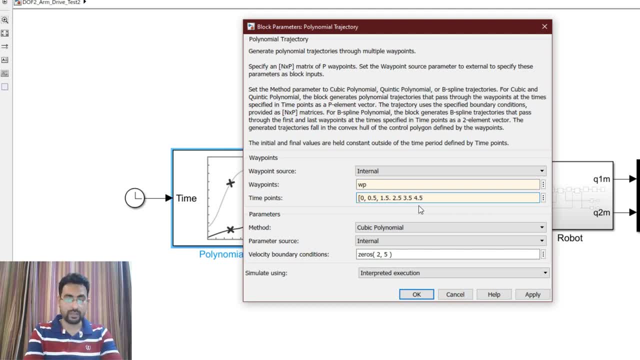 to complete the square in one more second, So I'm going to enter 4.5 once again. So that's it. These are the time points which I want my end effector to follow Under the parameters. I have three parameters over here. 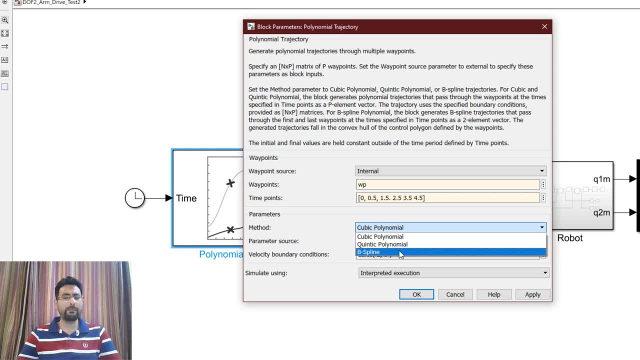 The cubic polynomial, the quintic polynomial and the B-spline. The simplest of these three parameters is the B-spline. In this B-spline you cannot specify the time points, because this polynomial trajectory block will generate one continuous B-spline that. 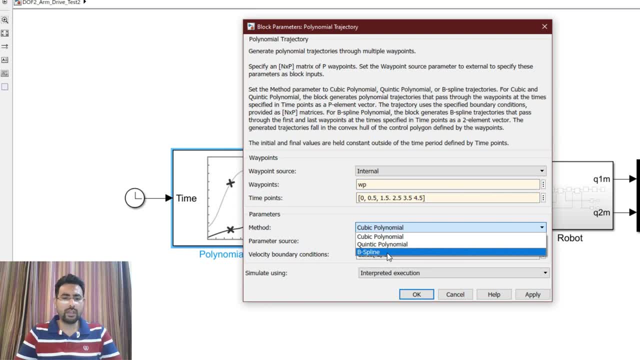 will start from the initial weight point, will try to reach the intermediate weight points and will end at the final weight point in the given time. So this thing won't be required by us because we want to go to each weight point In B-spline. there will be no guarantee. 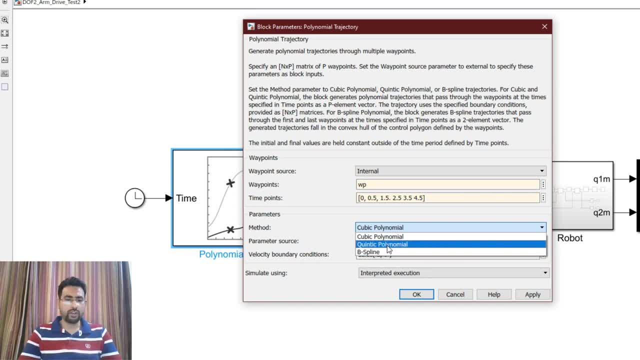 that certain weight points are going to be achieved or not. So we are going to go with either cubic polynomial or quintic polynomial. In cubic polynomial we have to define the velocity boundary conditions that. what velocity do we require when a certain weight point is achieved? 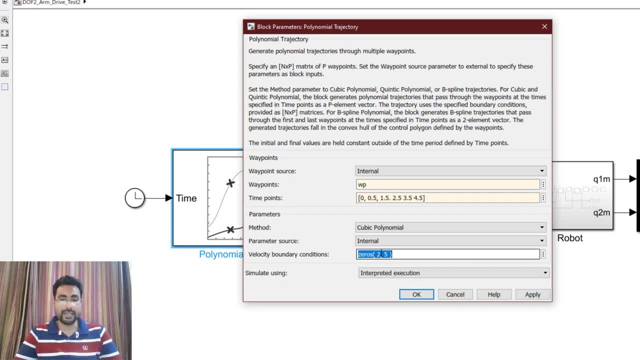 And we have to define the velocities in all x's, x, y and z-axis. So in z-axis we are not moving, so that can be 0. Whereas for x and y we have to define the velocities. But remember that if you approach a certain weight, 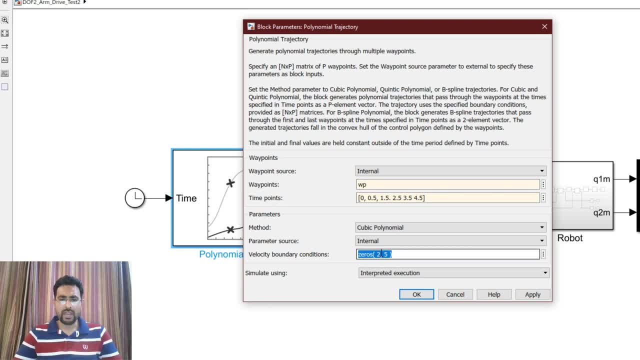 point through a non-zero velocity, then you can never make a 90-degree turn or a sharp turn. You have to stop over there. That is, you have to stop at the weight point, then change your direction and then move in the other direction. 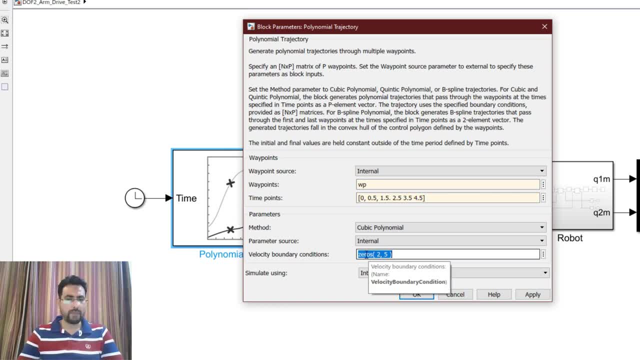 So if I will give 0s as all velocity boundary conditions, then I can draw the square perfectly. Otherwise, if I'm going to give any non-zero velocities, the square won't be drawn perfectly. So let's for the first time give a 0 velocity. 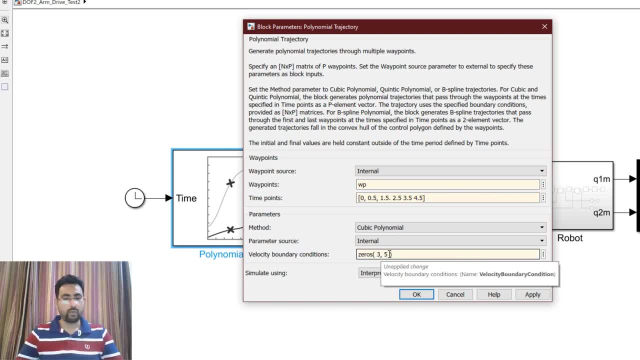 And then we will see that. what if we give a non-zero velocity? what is going to happen? So I have made it 3.. 6, because I have three x's, x, y, z, and I have six weight points. 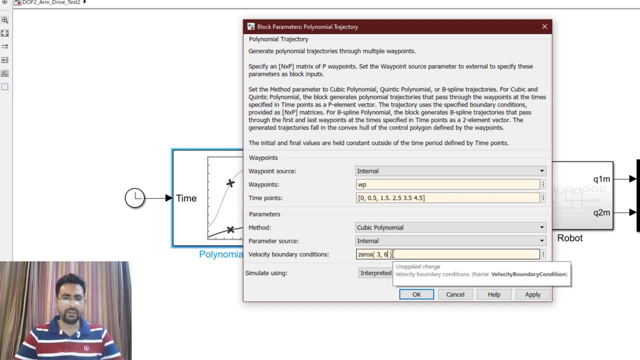 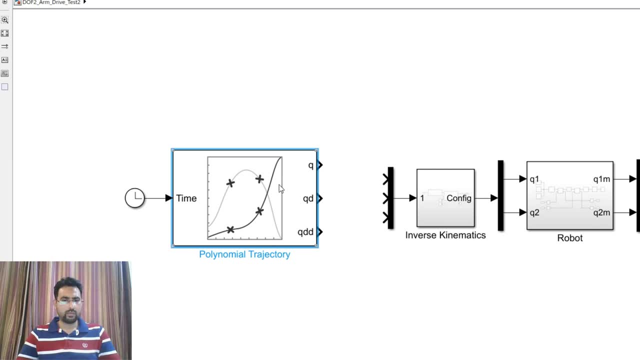 So I want my end effector to be at 0 velocity whenever it reaches a certain weight point. So that's it. This is all I have to do to generate the trajectory. So I'm clicking OK over here And this will generate the trajectory. 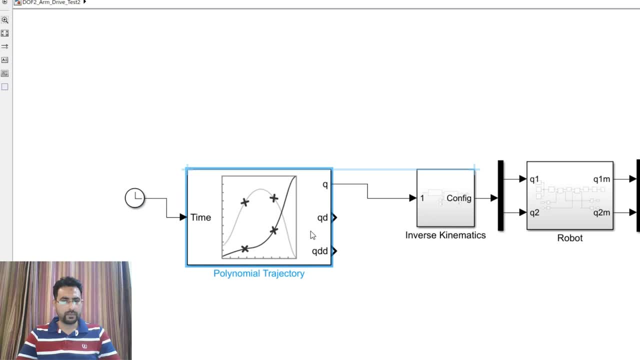 Now I need to provide this trajectory to the inverse kinematics block. So I'm giving it like this And if I want to plot or see that what trajectory I have generated, what are the velocities and what are the accelerations, I can simply use these plots to plot these things. 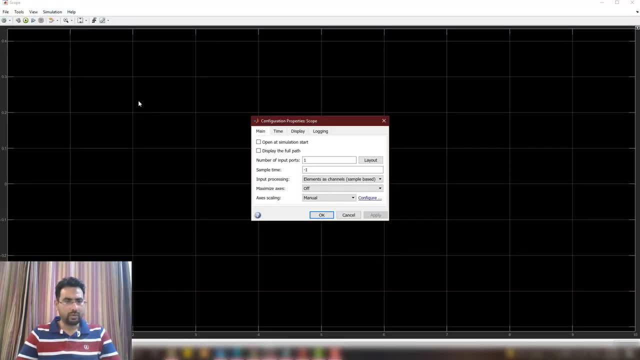 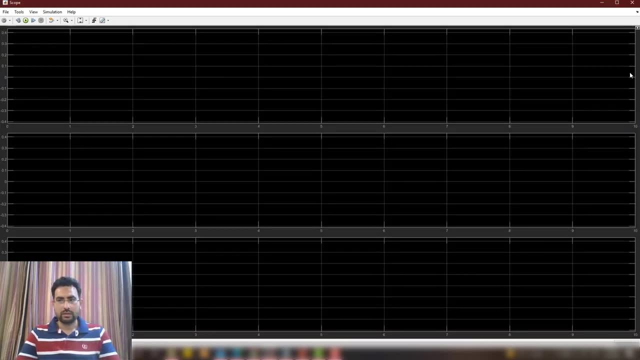 on the scope. So let me plot at least the trajectory and the velocity. So I'm going to change the scope from number of inputs from 1 to 3. And I'm going to choose this layout. That's it Now. in the first graph, the end effector position. 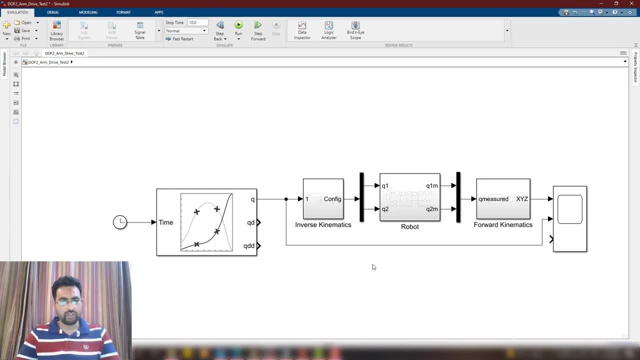 will be shown In the second graph the positions which are generated by the trajectory block. those are going to be shown, And in the last graph the velocities are going to be shown. I'm not concerned about the acceleration, so I'm going to terminate them using a terminator. 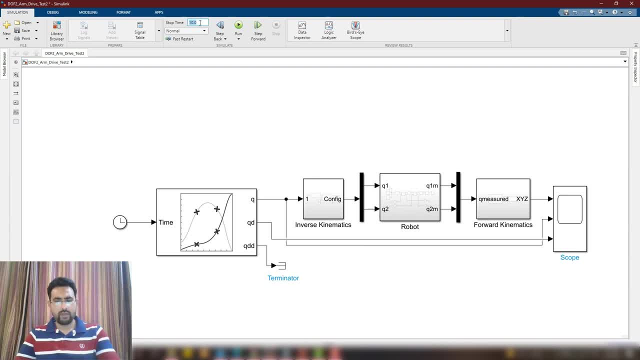 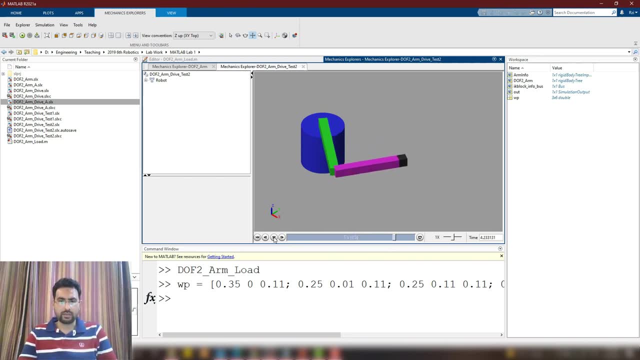 So this is everything we have to do Now. I just need to run it. So let me run it for five seconds only. So this is the complete simulation that we have. You can see that the manipulator is moving in a square. 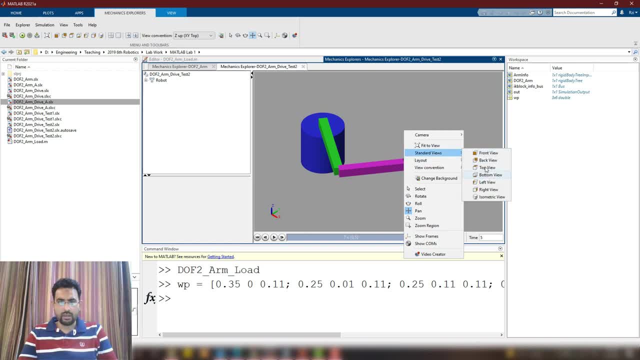 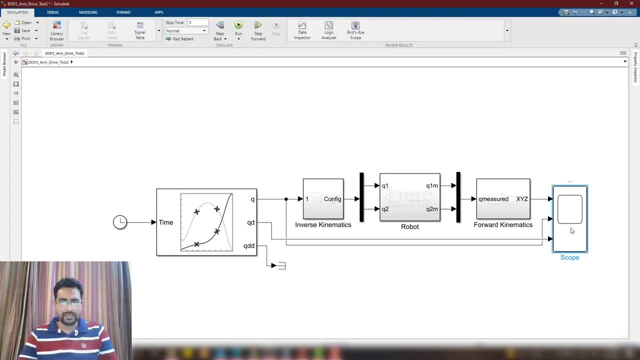 And, furthermore, if you change the view to the top view so that we can better see that, whether it is moving in a square or not, it can be seen that it is moving in a square. And if we want to analyze that, what are the velocities with which our manipulator is moving? 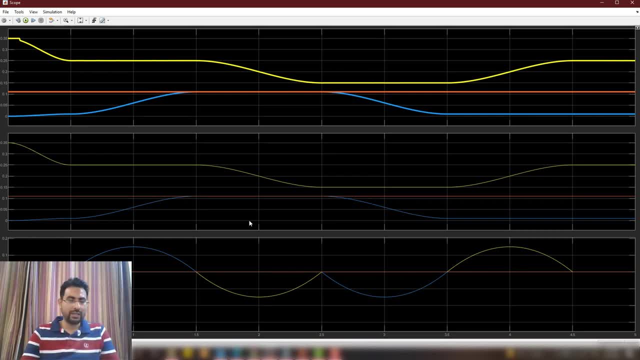 and what is the trajectory that the trajectory block generated? then over here we can see those things. The very first graph is the measured position of the x, y and z-axis of the end effector which the forward kinematics block was measuring. 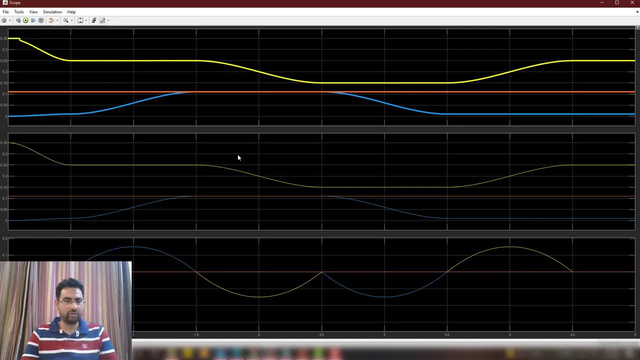 The second graph shows the trajectory that was generated by the trajectory generation block, And this third graph shows the velocities in x, y and z-directions. Yellow is the velocity in x-direction, Blue is the velocity in y-direction And red is the velocity in z-direction. 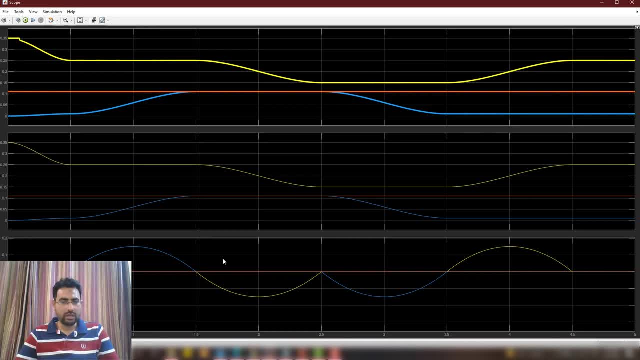 As the manipulator is not moving in z-direction, so we don't need the velocity in z-direction. That is why you are seeing a flat line, Whereas for x and y-axis you can see that how velocity is increasing, then decreasing and then increasing again. 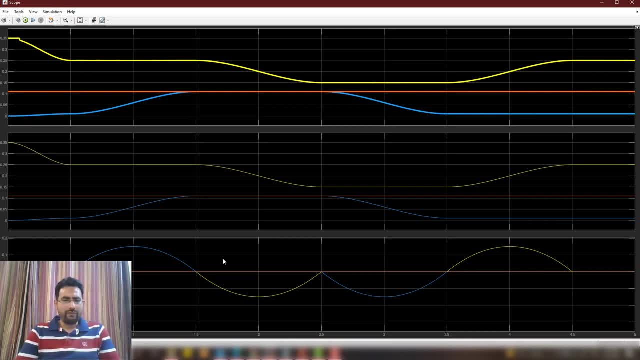 and all these things are happening. So what if we wanted to increase the speed of our manipulator? That is, we want to trace the square in a much faster fashion, or in a much slower fashion, maybe? So all we have to do is we have to change the time points. 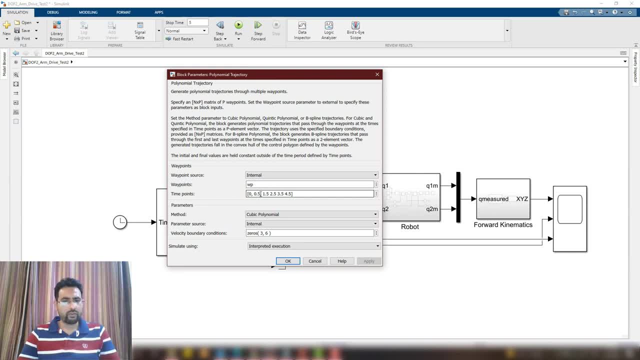 over here. So now, let's suppose we want the end effector to reach the starting point, that is, the first corner of the square, using 0.5 seconds. Then each subsequent corner of the square should be reached by, let's suppose, 0.2 seconds only. 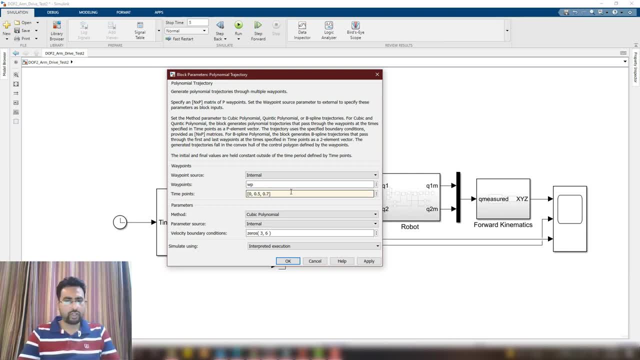 So at 0.7 seconds the end effector should be at the second corner, Then at 0.9 seconds it should be at the third corner, Then 1.1 seconds at the fourth corner and 1.3 seconds. 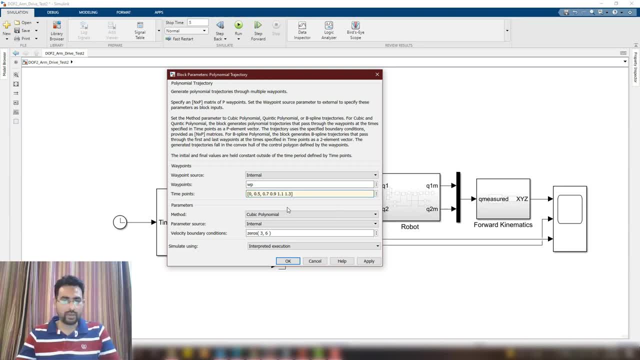 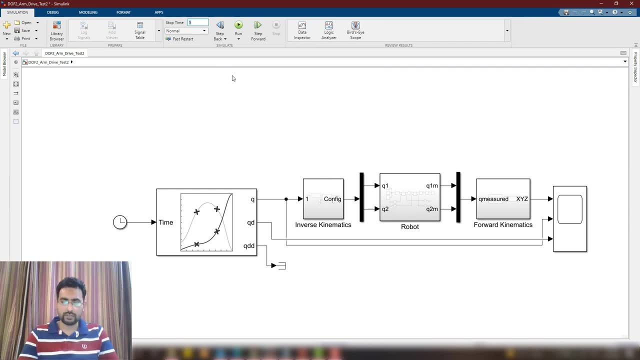 back at the start. So all I need to do is I need to change these time points, and that's it. I'm going to rerun the simulation once again. This time I won't be needing 5 seconds, I only need to simulate it for, let's suppose, 1.5 seconds. 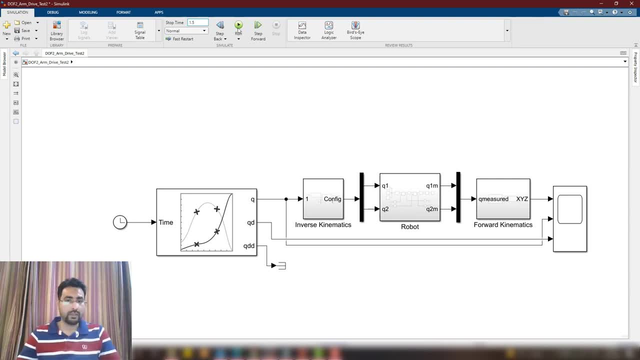 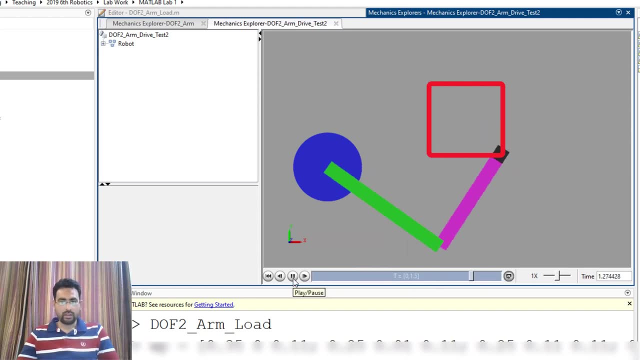 because I know that at 1.3 seconds my trajectory would be completed. So this is the simulation result now, which I think is going to be a lot faster. You can see that how hastily it moves in a square. The initial approach of the square is in 0.5 seconds. 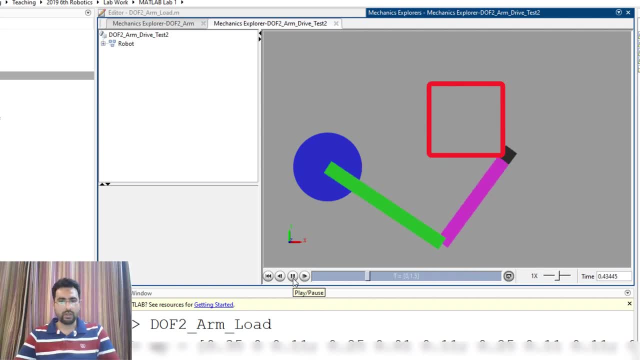 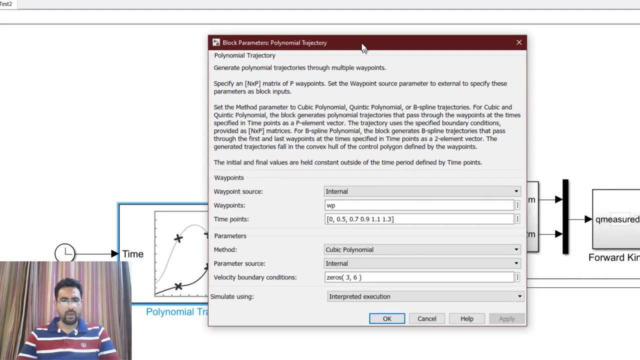 Then each line segment of the square is drawn in 0.2 seconds only. So it is quite fast, And all we had to do is that we gave the changed time points. Now let us experiment that. What if we don't give non-zero velocities at the waypoints? 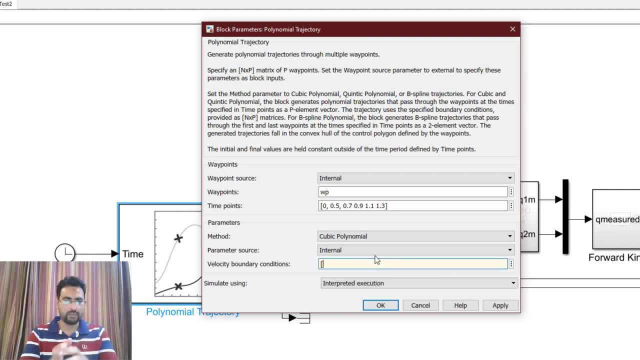 So for that, the initial waypoint should be at zero velocity, because our robot is starting from that point. I'm going to give x direction, I'm going to give the same velocity at the initial waypoint as zero, Then at the next waypoint I want my end effector. 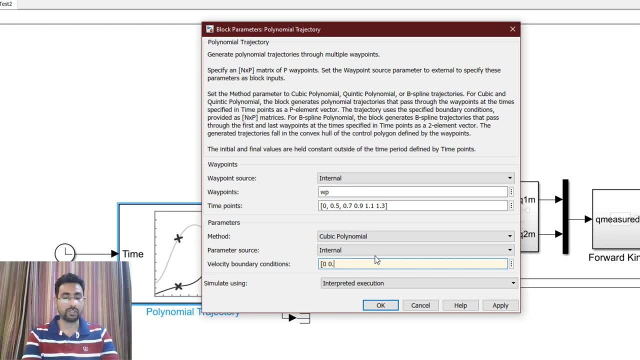 That is the first corner of the square. I want my end effector to have a velocity of, let's suppose, 0.1.. Then at the second corner, I want 0.1 velocity, then 0.1 again, 0.1 again. 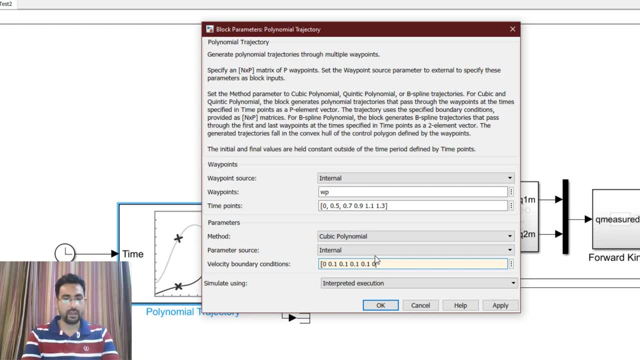 And at the last waypoint, I want the end effector to have, let's suppose, zero velocity this time, so that it will stop at the end. These are the velocities in x direction. Same velocities for the y direction And for the z direction. I don't want. 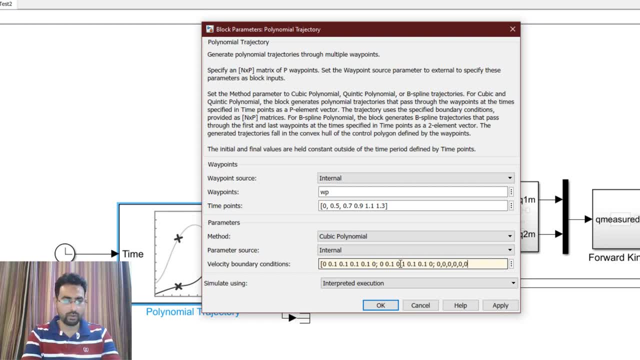 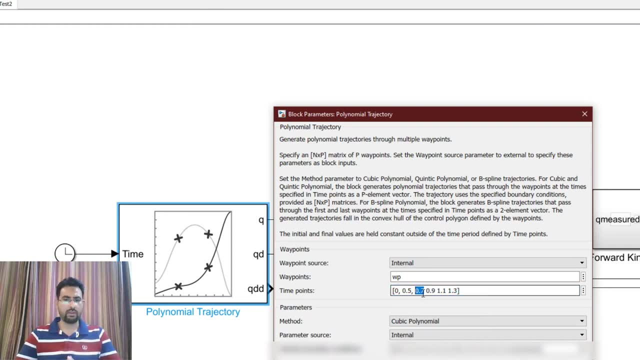 any velocities. so I'm going to give six zeros because I'm not moving in the z direction. So that's it Now. let us see that what happens. Moreover, let me change these time points back so that our manipulator doesn't move so fast. 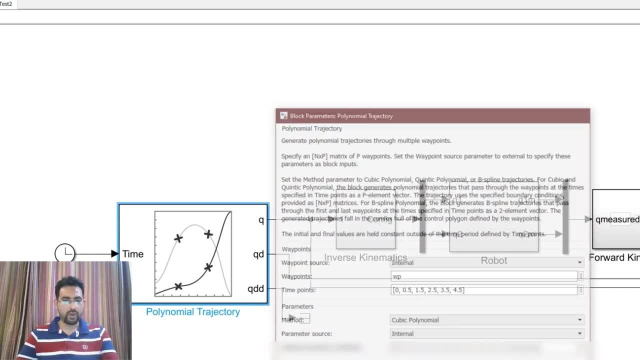 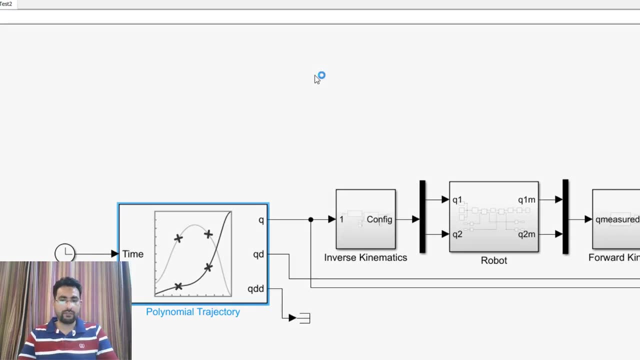 I'm going to change them to 1.5.. So now let's see what happens. I'm going to now run this thing for five seconds, because I know that the trajectory would be completed in 4.5 seconds, so five seconds would be sufficient. 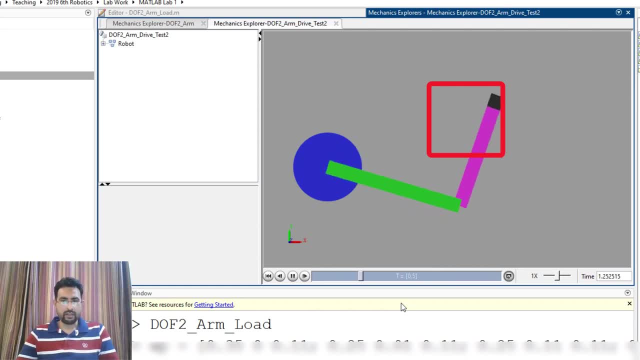 So now see that what is happening? because we wanted the end effector to keep on moving. It doesn't stop at the waypoints, And at the waypoint it should have a velocity of 0.1 meters per second. Therefore, the end effector is not tracing the square quite. 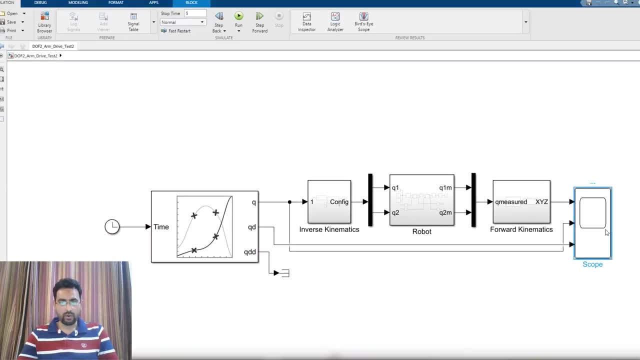 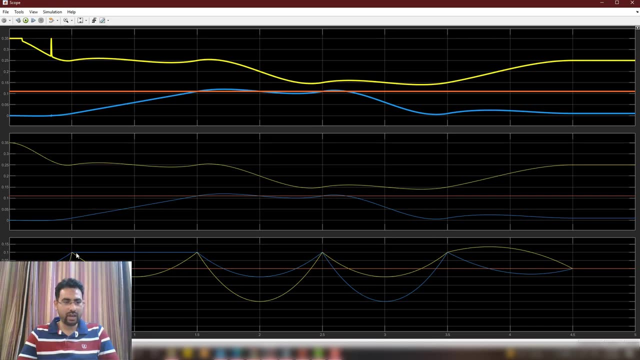 perfectly. If we see that thing on the graph, we'll see that what is happening Over here. we can see that the velocities at the waypoint- this is the first waypoint Over here- both velocities in x and y direction- are 0.1.. 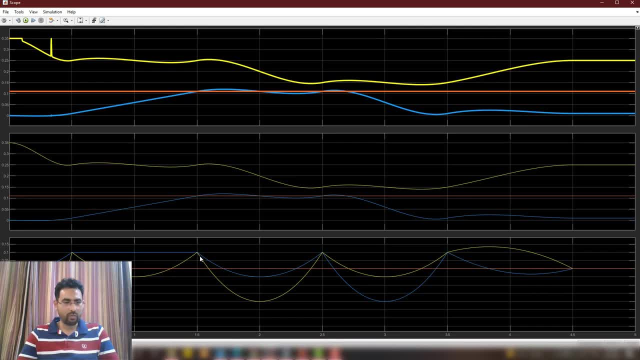 Then over here at the second waypoint, the velocities are 0.1 meter per second once again. Then this is the third waypoint, the fourth waypoint and the fifth waypoint- The first one is over here, So in total we are having six waypoints. 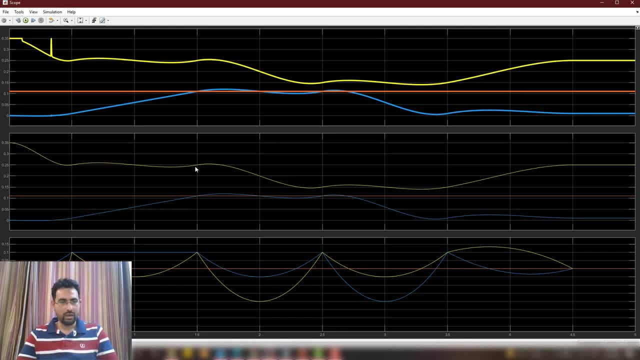 But look over here that nothing over here is smooth, because if we want to have a velocity of 0.1 at this point, then we cannot approach this point and change our direction abruptly. So we have to approach this point from some other trajectory. 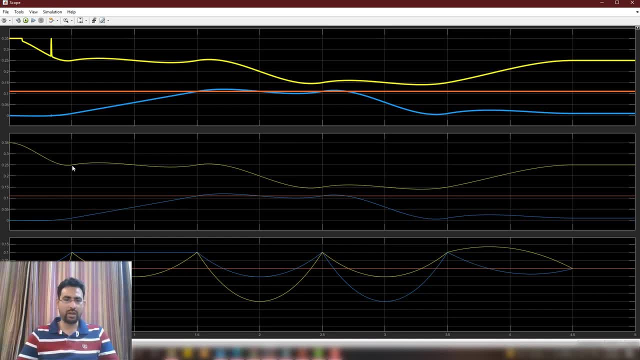 so that we can move through this point, that is, achieve this waypoint but still have some velocity. This is happening at all these waypoints, So that's why we are not going to trace the square perfectly If we increase this velocity to a higher value. 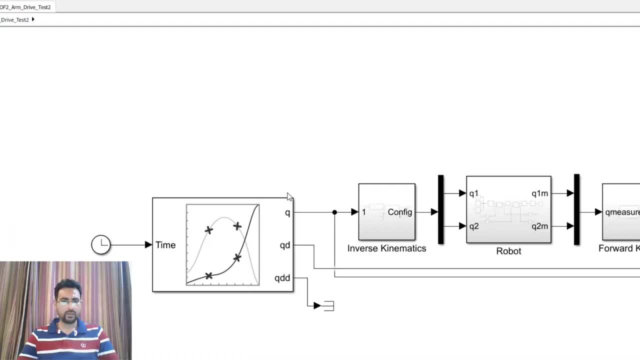 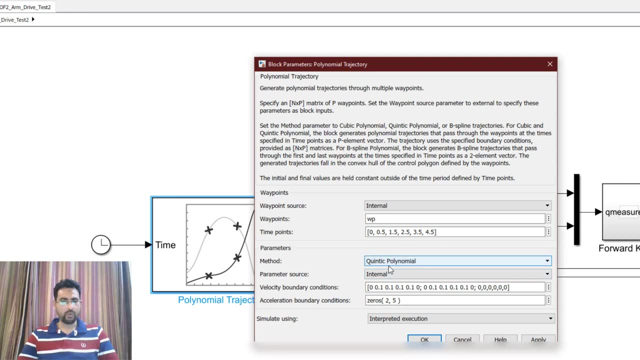 then you will see that the tracing would become much more poor. So another thing that you can do with this polynomial trajectory is that you can use a quintic polynomial over here, And if you are going to use a quintic polynomial, then you will have an option of specifying acceleration boundary conditions. 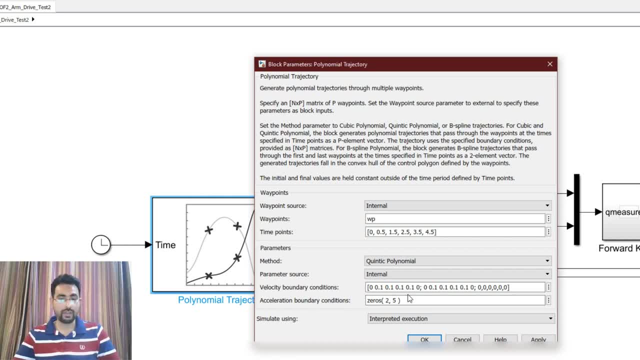 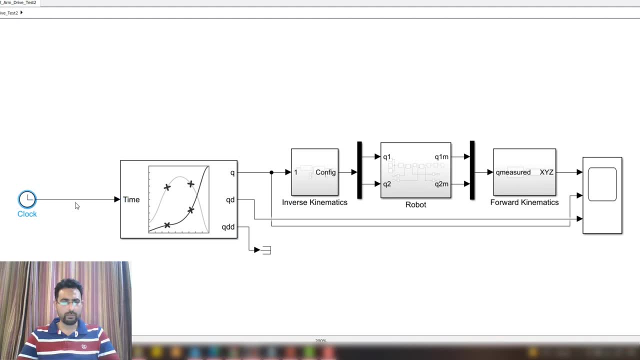 that what acceleration at waypoints your end effector should have. But that would become quite complex for the time being, so I'm going to skip this thing. So that's everything which I wanted to talk about: the polynomial trajectory And the next block which I'm going to talk about. 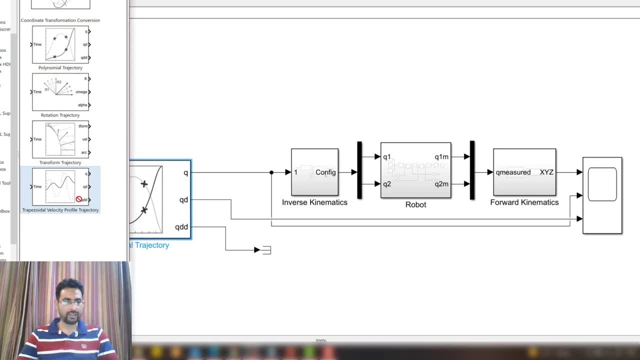 is the trapezoidal trajectory, So I'm going to drag this block over here, And now I'm going to delete this thing. I don't need this one anymore. I'm going to place this trapezoidal velocity profile trajectory over here. 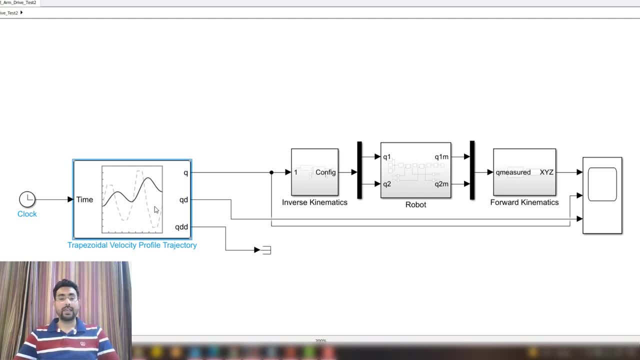 What trapezoidal velocity profile trajectory means is that it is going to move with a constant acceleration, achieve a certain velocity, then move with that constant velocity for some time, and then going to decelerate once again. This thing is very useful. 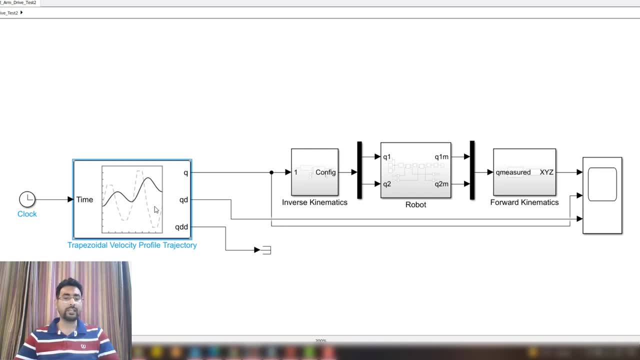 if your robotic manipulator wants to move in linear motions, That is, it wants to track the velocity, That is, it wants to track the velocity. And in our case, we want our manipulator to move in a straight line, because the square is the form of four straight segments. 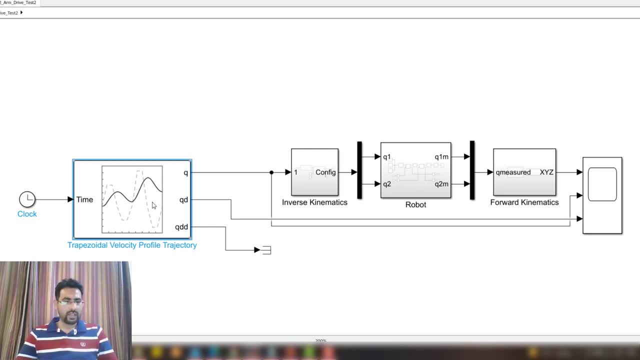 So this thing is going to be perfect for us. So, once again, the input for this block is time, which I have connected already, And the output of this block are once again going to be the positions: the x, y, z trajectory positions. 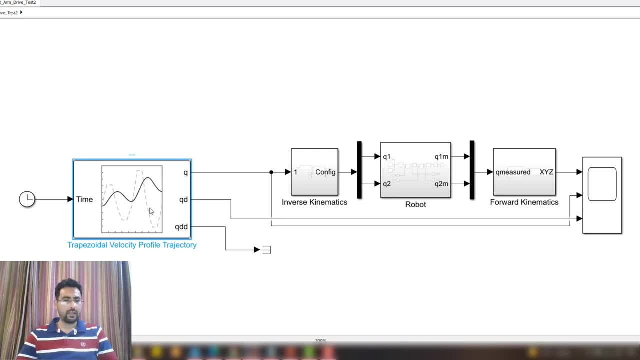 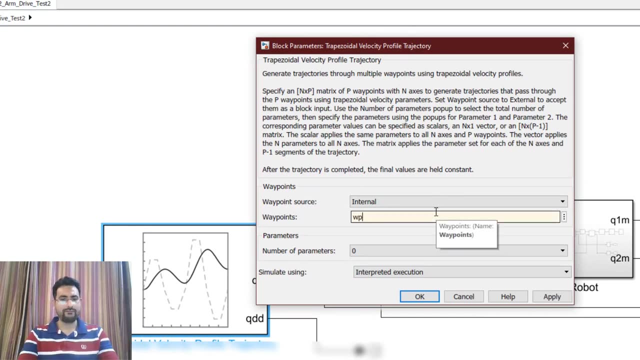 the x- y z velocities and the x- y z accelerations. But inside this block the things are a bit different. The very first thing is once again the same, That is, the waypoints. I'm going to supply the same waypoints over here. 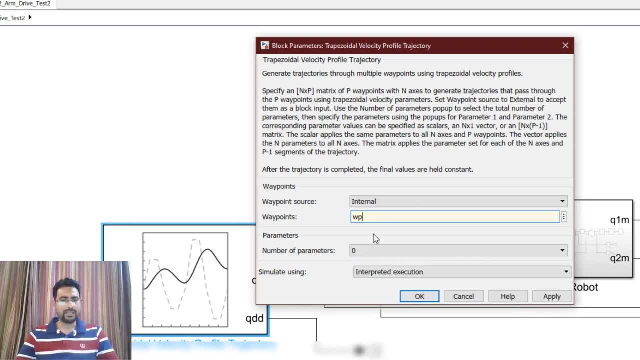 which is WP. I have already created that variable. And the second thing is the parameters. If I won't specify any parameters, then this block will automatically generate a trajectory which will have a trapezoidal velocity. That is, the end effector is going to move in a trapezoidal velocity fashion. 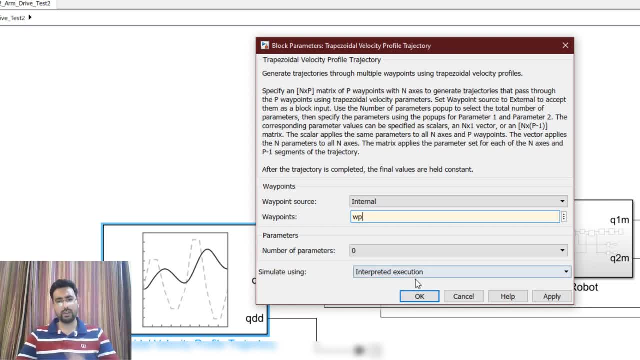 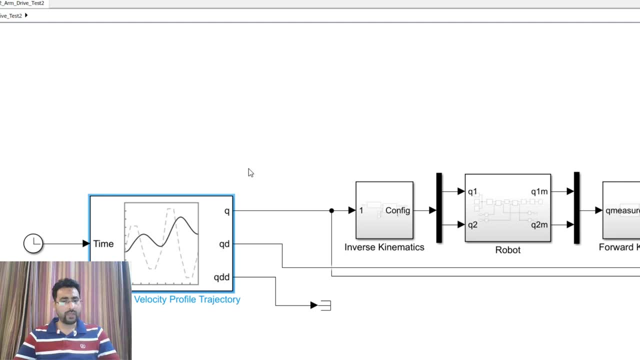 and will achieve every waypoint after one second. So let me first run it and see what is happening. Keep one thing in mind over here: that the trapezoidal velocity profile trajectory will make sure that the end effector achieves a zero velocity at every waypoint. 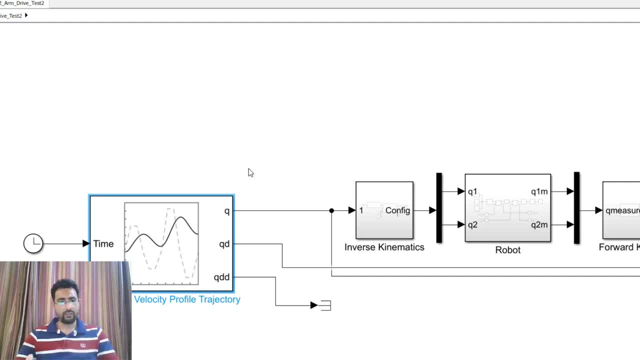 So we are going to move in straight lines, then reach the endpoint or the waypoint, then stop over there, then move in some other direction, So we don't need to worry about the velocities at the waypoints. So what's going to happen over here is that. 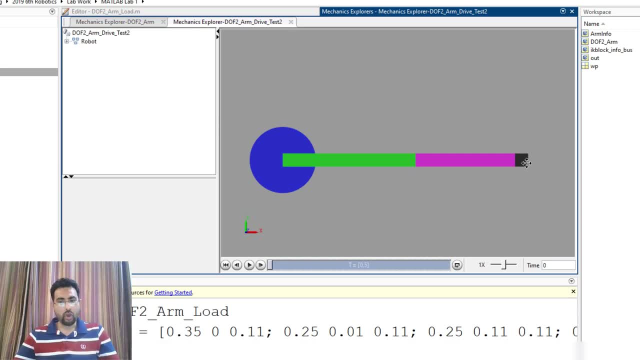 the end effector is going to move to all the waypoints and then stop over there and then move towards the next waypoint. The stopping will not be that visible because immediately it is going to move to the next point, But it is going to approach a certain waypoint. 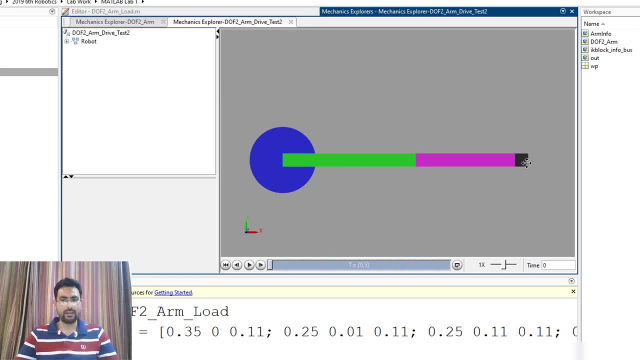 slow down there and then approach a zero velocity, then speed up once again in the other direction and then move towards the other waypoint. And this is what naturally we do If we are drawing a straight line. we start from a point, our hand accelerates. 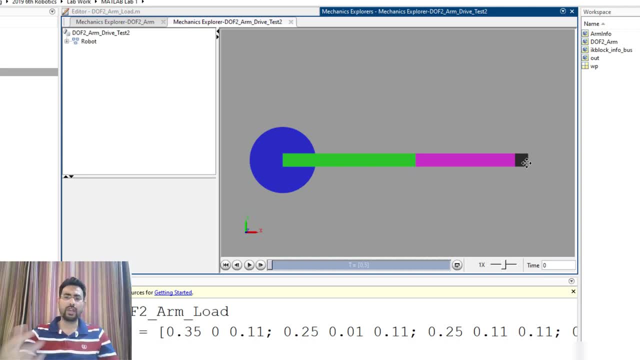 then reaches a constant velocity and then, as we are approaching the other endpoint or the waypoint, we slow down and then we approach that point with a zero velocity, change our direction and then start drawing the line in that direction. So this is what is happening over here. 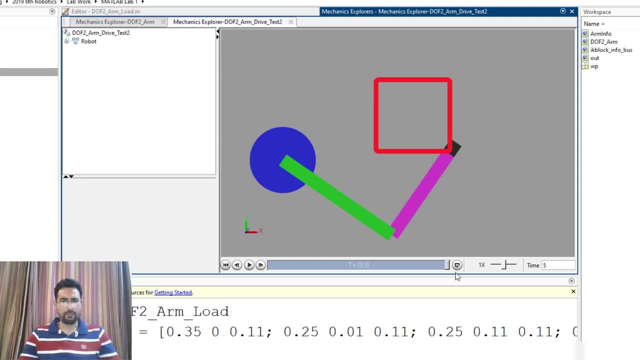 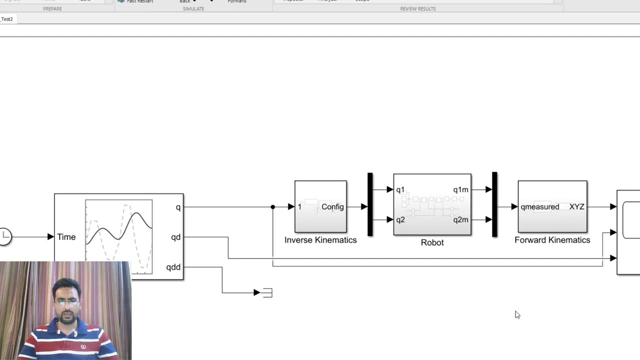 You can see that it is a much smoother thing or a much natural thing which is happening. We are approaching the waypoints very smoothly, We are stopping there and then moving towards the other side. If we see the velocity profiles, then you will be able to see that. 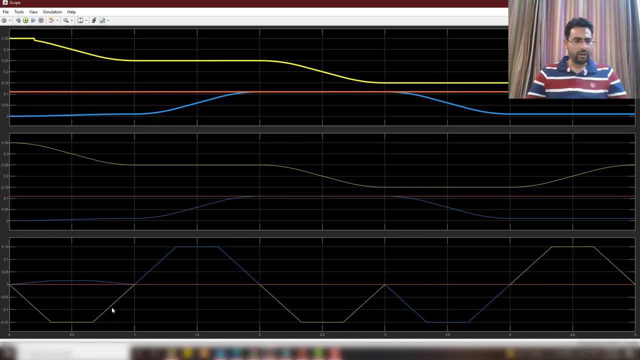 how velocity is changing In the x direction. over here this yellow line is showing the x direction. So in the x direction we are accelerating first, then achieving a constant velocity, and then decelerating once again to stop at the first waypoint. 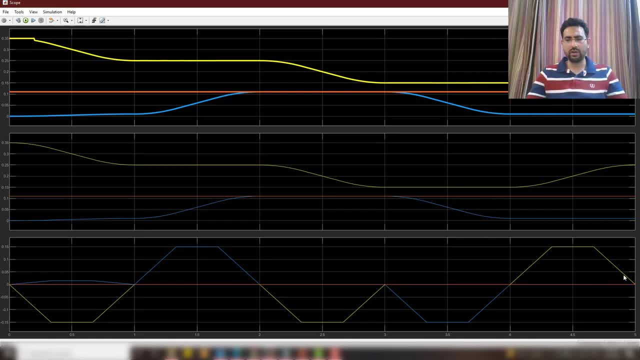 Then this is the second waypoint, third waypoint, fourth and the fifth. If zero, one is of course the first waypoint. that is why we are having six waypoints. So this is what happens, And over here you can see the trajectory. 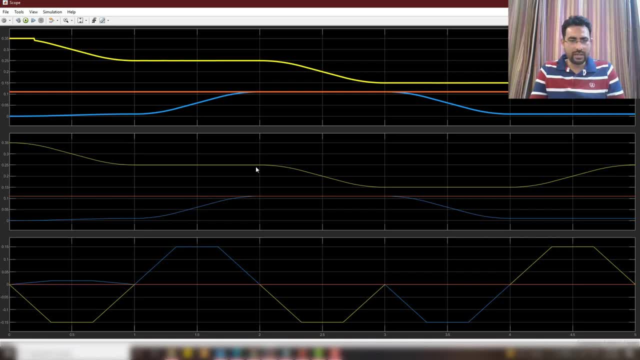 that how it is changing. We are achieving the waypoints. that is this point, this point and all the other points. But as soon as we approach a certain waypoint, the end effector slows down, That is, its velocity is slowing down. 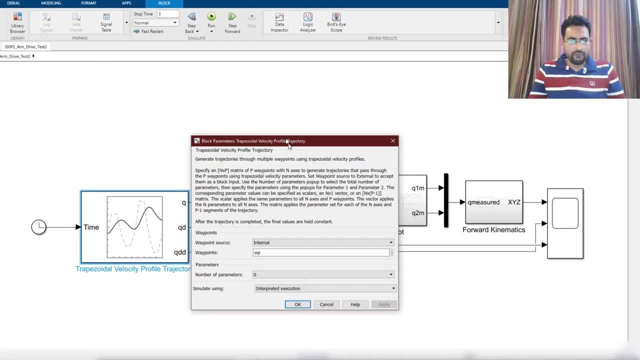 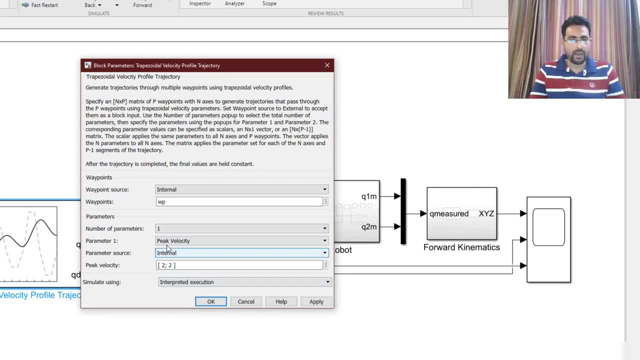 Now let us see that. what other options in this block do we have? So if we want to specify parameters, then there are two options. We can either specify one parameter or two parameters, And if I select one, so these are the four parameters. 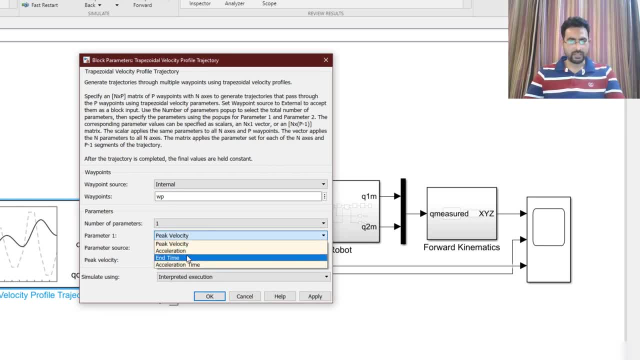 that I can change if I select the number of parameters as one. The first one is the peak velocity, that in trapezoidal velocity what is going to be the peak velocity. The second one is the acceleration, because as the velocity is increasing, 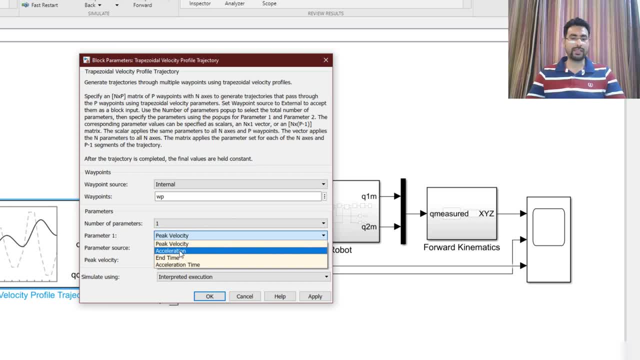 and then it is decreasing. so what would be that acceleration and deceleration value? The third one is the end time, that is, what time it requires for each segment of the trajectory to end. And then the last one is the acceleration time. 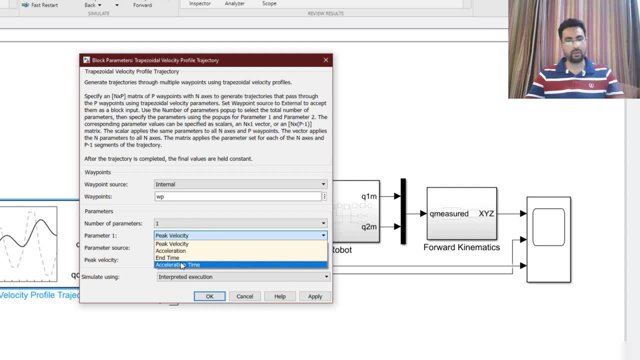 that is, for how long acceleration should be there and correspondingly deceleration as well. So let me choose end time over here, And then I can specify that at what time each segment should end. Right now it is one. That is why it was taking one second. 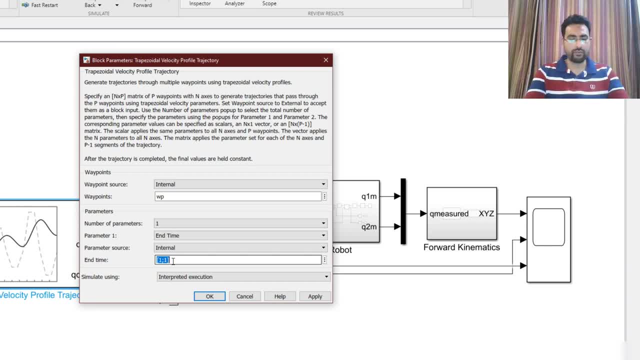 to complete each segment, But I can change that to, for example, 0.5.. Now each segment would be completed in 0.5 seconds, But if I want separate segments to complete at a separate time interval, then I can change that. 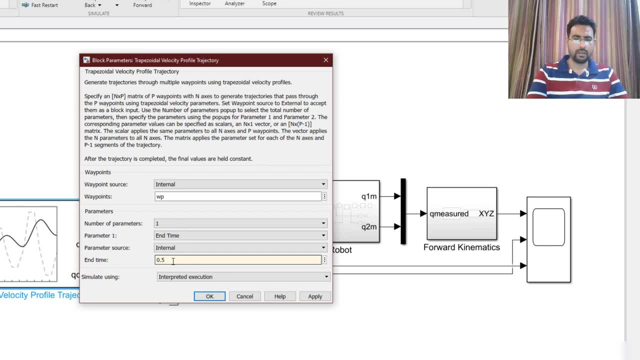 and I can specify that thing over here. For example, I want in the x direction, I want the segments to end at, for example, the first one in 0.5 seconds, the second one in one second, then in one second. 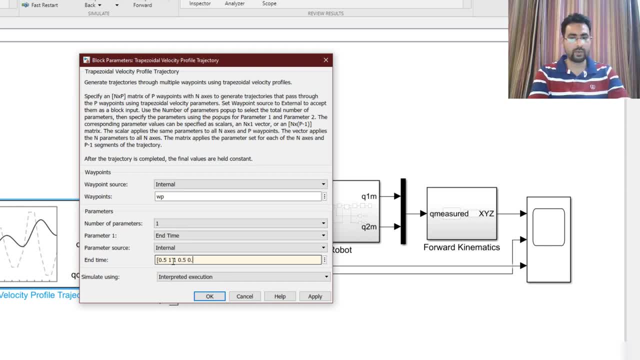 then in 0.5 seconds again, and then the last one in 0.5 seconds once again. So my first segment is going to end in 0.5 seconds, then the second segment, that is, the first vertical line of the square. 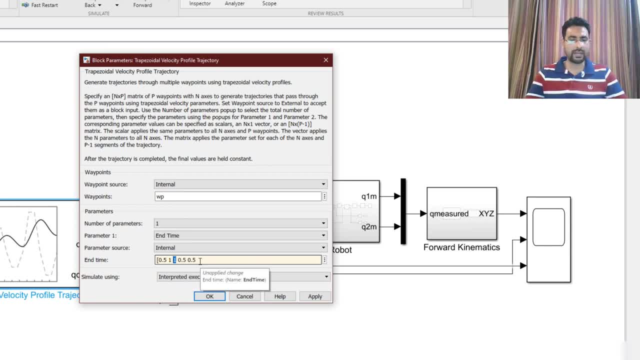 in one second, then the second one once again in one second, then the third and the fourth line would be completed in 0.5 seconds. Note that I have six waypoints, so I'm going to have six minus one segments. So, for the sake of simplicity, 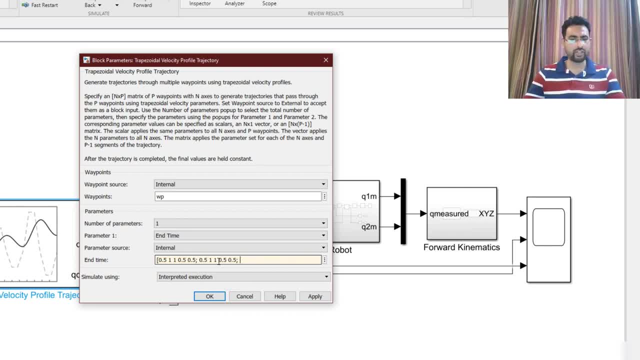 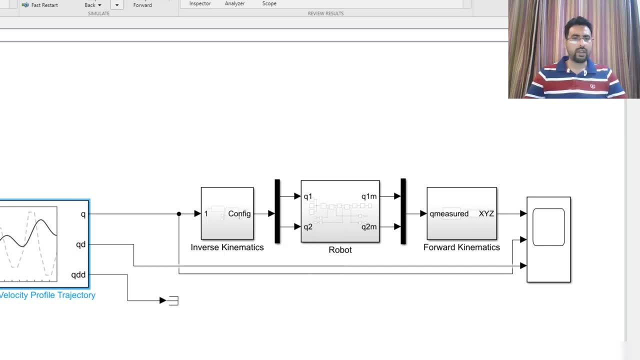 I'm going to use the same n times in y direction and in z direction as well, Although I'm not moving in the z direction. but I need to specify some points over here. So now let me run it and see that what happens. 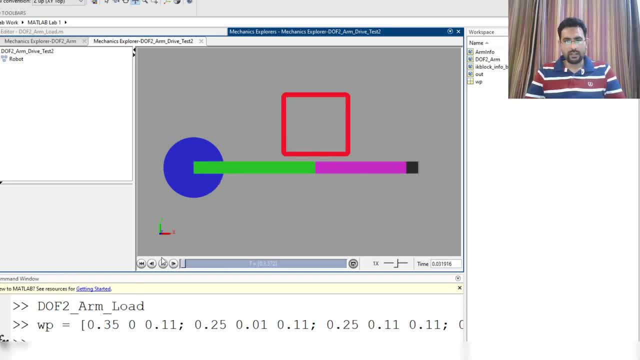 So this is what we have. You can see that the first two segments of the square are being drawn slowly because we specified one second for that, and the last two segments are being completed quickly because we specified 0.5 seconds for that. If we see the trajectories in the scope, 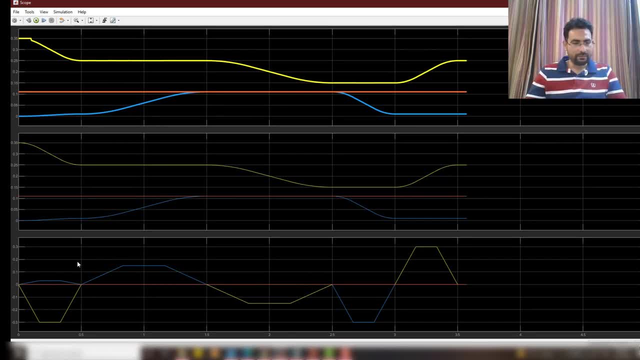 then we would be able to see that these first three segments are being completed in 0.5 seconds, then in one second and then once again in one second. So these two straight lines of the square are being completed in one second, and then the next two lines. 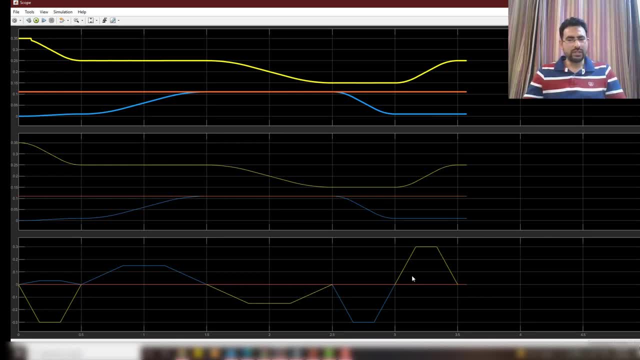 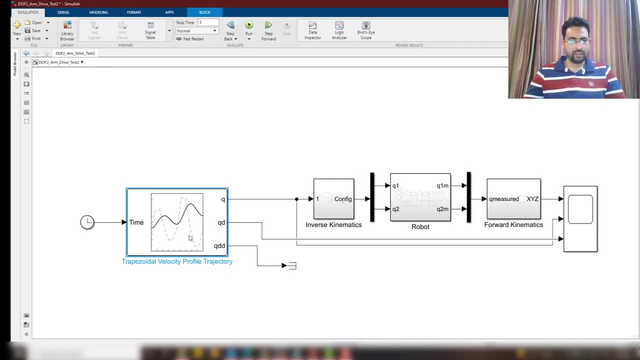 are being completed in 0.5 and 0.5 seconds. So you can see that how simply we can generate trajectories and how efficiently we can control different aspects of those trajectories If we come back to this trapezoidal velocity profile trajectory block. 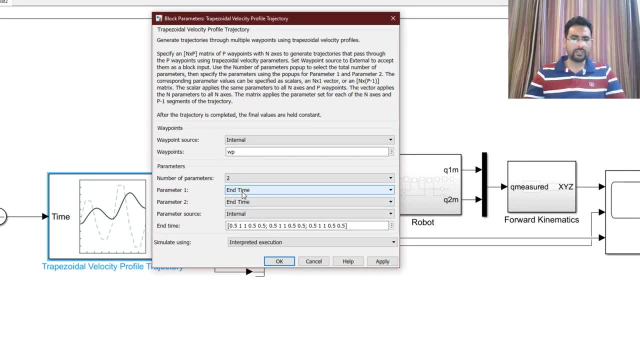 if we use two number of parameters, then out of these four parameters we can specify two of them, That is, we can control two of them. I can control the end point and I can control the peak velocity as well. But be advised that certain end times. 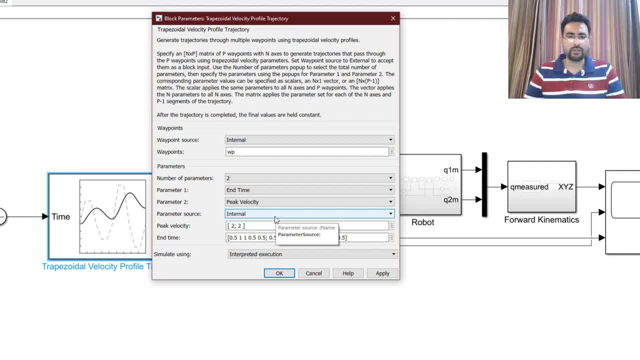 and peak velocities might not agree with each other, So the points that you have specified might not agree with each other. That is, you cannot achieve a certain peak velocity with a certain end times which you have specified. So you have to be careful about the choices. 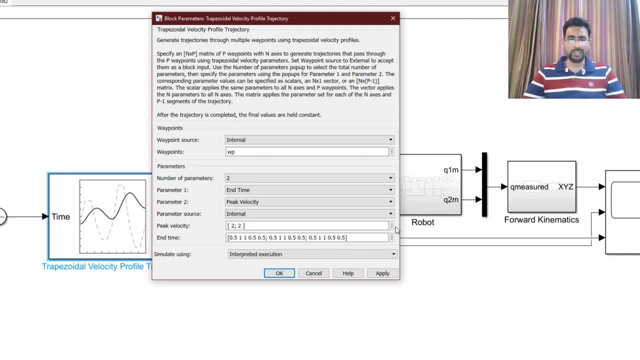 So that's everything which I have for this video. You can use these blocks to generate trajectories. You can control the velocities, the accelerations at the end points. You can simply specify the V points and these blocks are going to generate the trajectories.